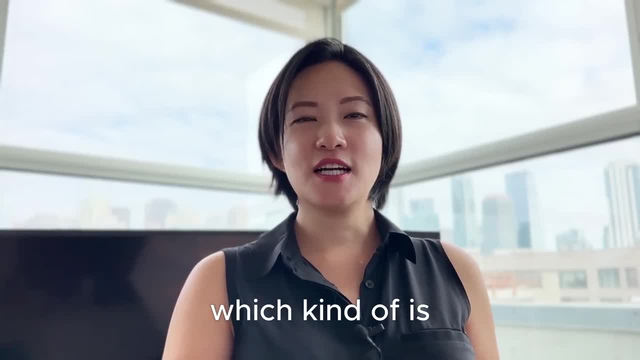 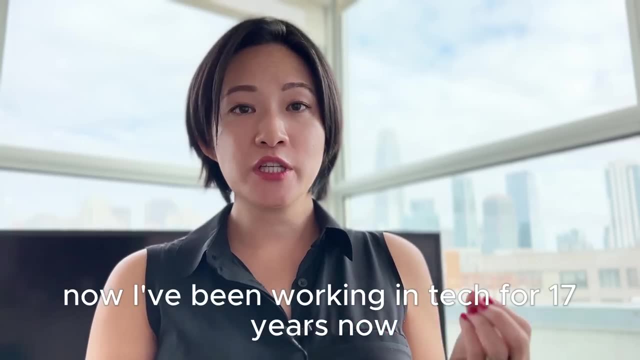 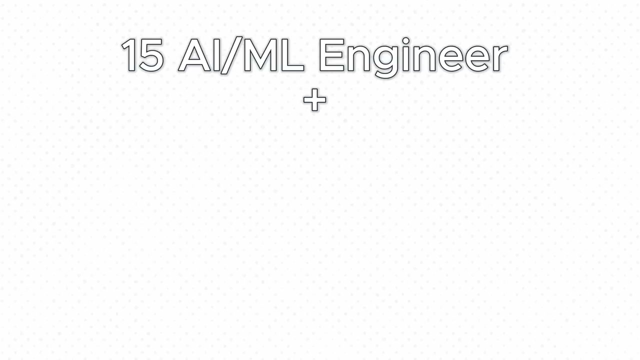 of like deciphering a secret code, which kind of is. I guess It is a common challenge in the tech world. trying to decode the lingo Now, I've been working in tech for 17 years now so I can help you translate this. Here's a breakdown. I looked at 15 AI ML openings, so 12 senior roles and 12 junior. 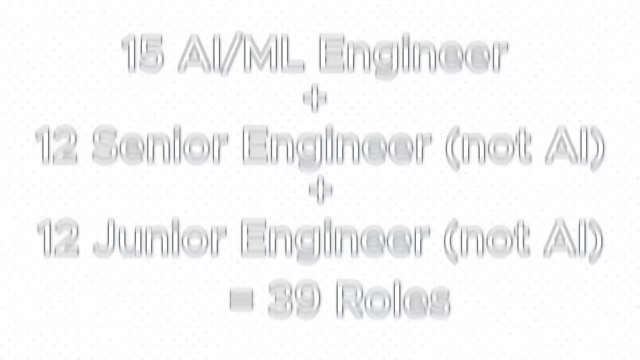 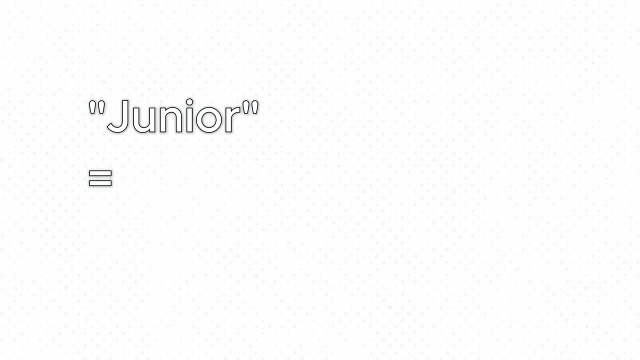 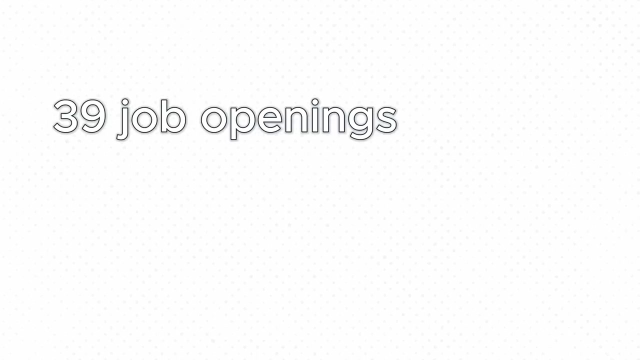 postings outside of AI, slash ML, and when I say senior roles, I had the word staff or senior in the title and then the junior roles had words like entry junior or new grad, but not AI or ML. In this batch of 39 positions, there were 1125 applicants and, as a premium LinkedIn user, 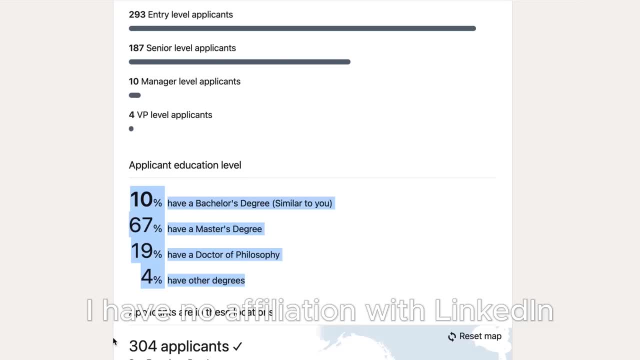 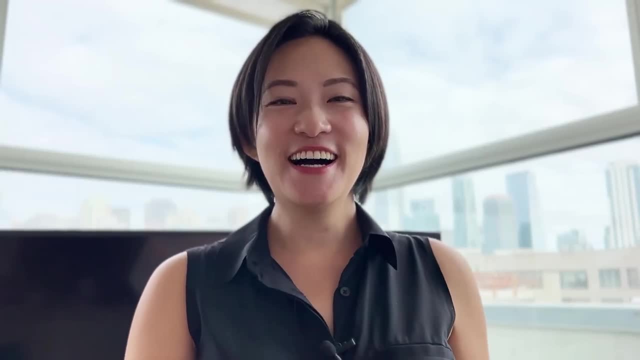 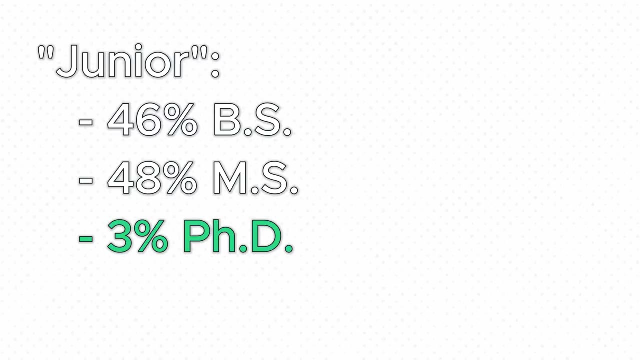 this data comes to me as a feature. I have no affiliation with LinkedIn, I just pay to use this feature. So what is the outcome? Drum roll please. Among junior roles, about half and half had bachelor's and master's degree and three percent had PhDs. Senior roles were about the same, except. 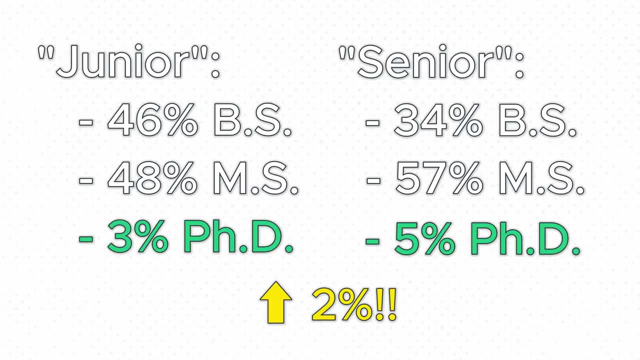 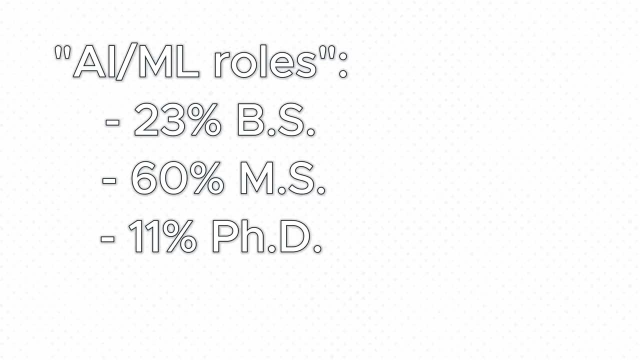 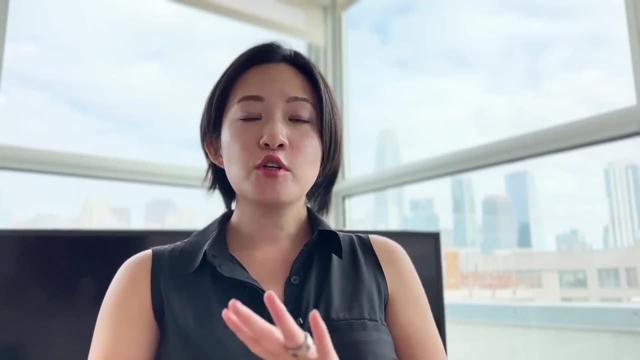 five percent had PhDs, so two percent more than the junior roles. Now AI slash ML roles on average of about a quarter had a bachelor's degree, while over half had master's degree and eleven percent had PhDs. Of the 24 non-AI ML junior and senior roles, only two explicitly mentioned the terms. 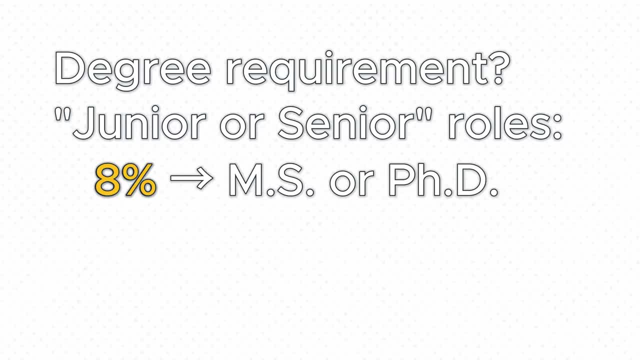 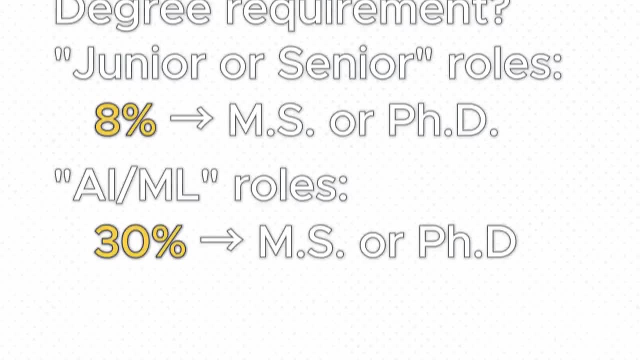 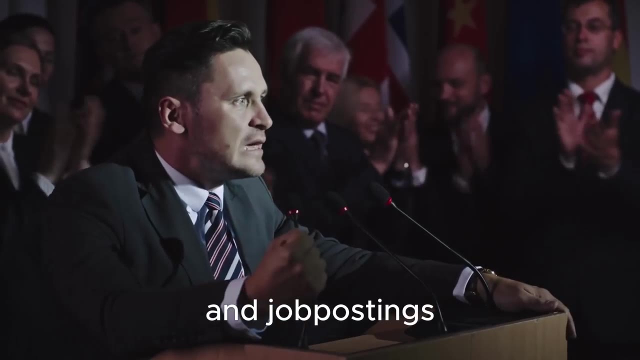 MS or PhD, which is about eight percent. In contrast, 30 percent of AI ML positions mentioned either MS or PhD in the qualification section. I know it's confusing. Yes, we could discuss the need for standardized titles in job postings, but that would involve a long-term shift. 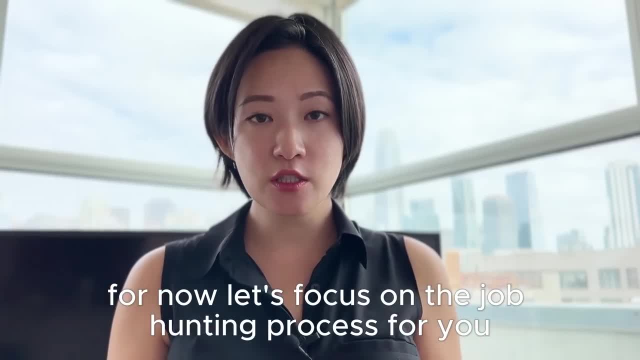 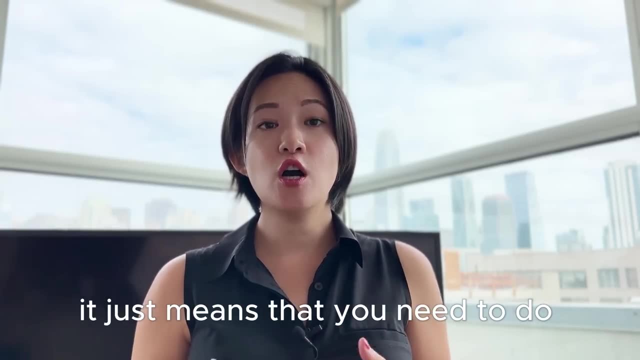 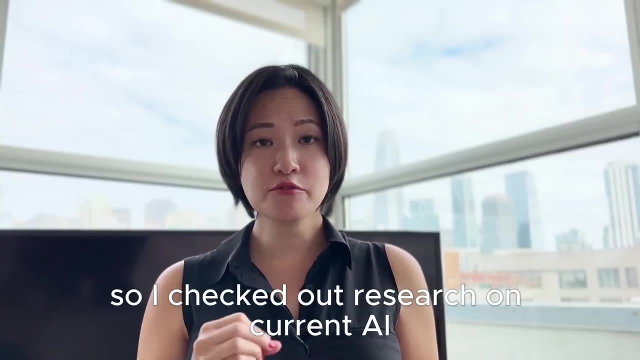 in the industry as a whole. For now, let's focus on the job hunting process for you. If you are actively job hunting now, it just means that you need to do a lot of reading. My research was on a small sample size- 1125 applicants- So I checked out research on current 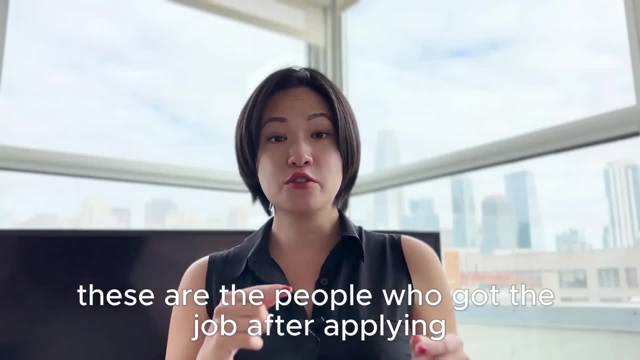 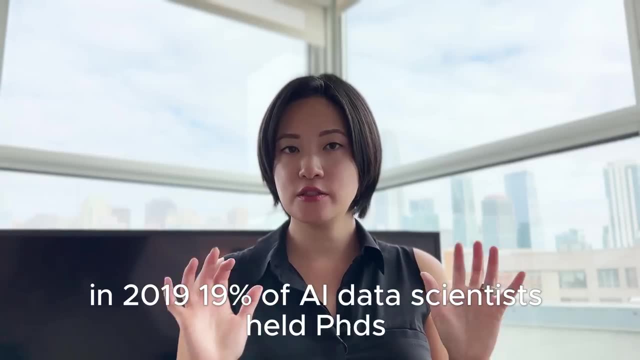 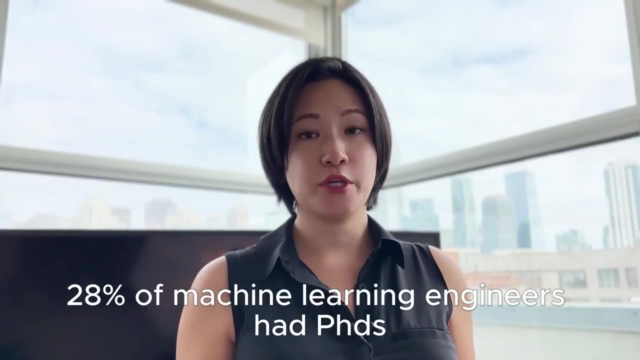 AI slash: machine learning engineers with PhDs. These are the people who got the job after a applying job in 2019.. 19% of data scientists held PhDs. In 2021 LinkedIn report, 28% of machine learning engineers had PhDs. Also, the AI index report from 2021 notes 45%. 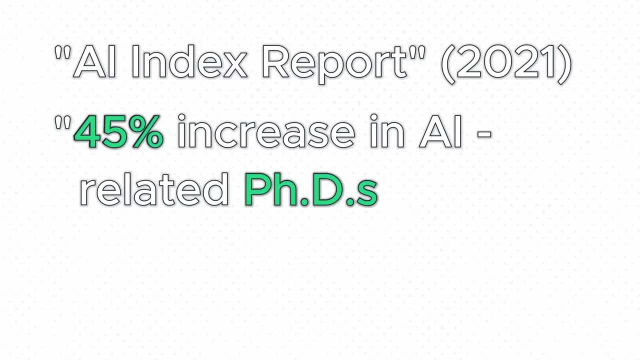 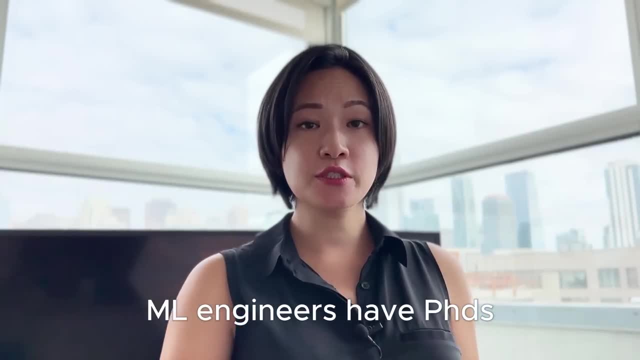 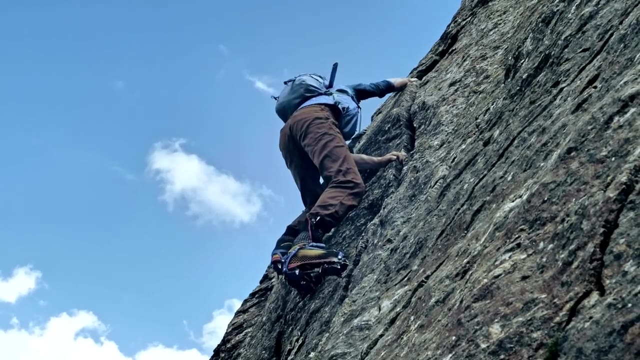 an increase in AI related PhDs granted from 2018 to 2019.. So it only makes sense that more AI machine learning engineers have PhDs, since more PhDs are applied and they have PhDs. people graduating PhD do it in AI and machine learning. Imagine climbing the Everest in sandals. 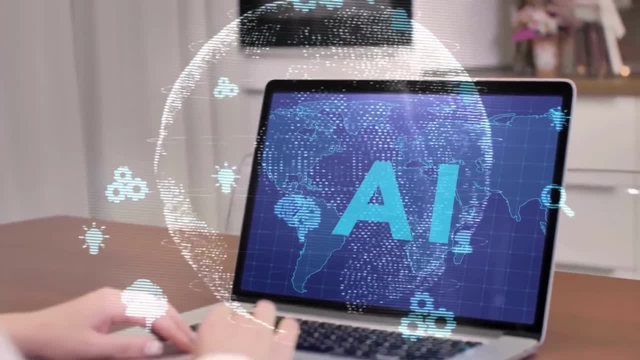 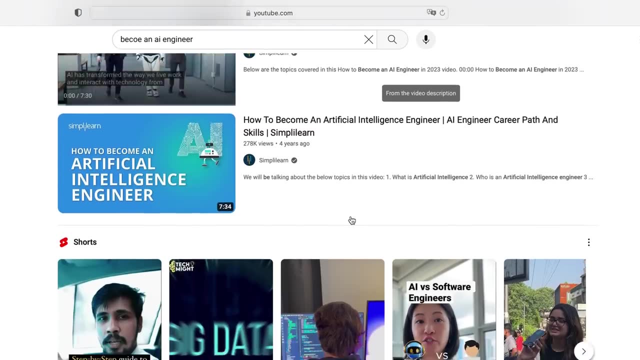 with no preparation or tools. That's kind of like trying to become an AI or machine learning software engineer with no experience overnight- And I have seen these videos or gurus claiming that you can become an AI or machine learning engineer overnight. Then you apply to hundreds of these roles and you 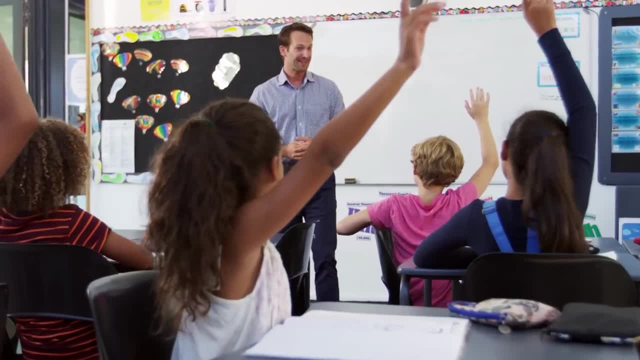 can't land a single interview. Then you ask me: what am I doing wrong? Well, you're on the wrong path. my friend And I get it. That's where the future is going. So here's the secret, If you have. 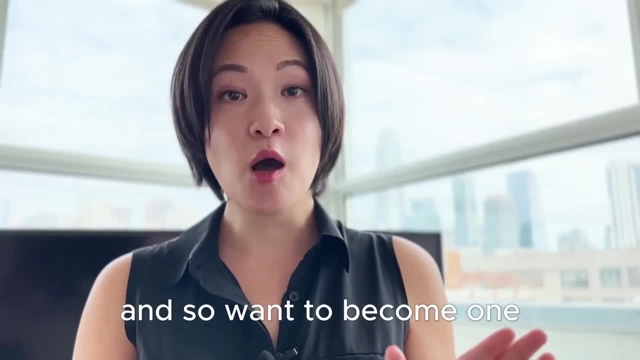 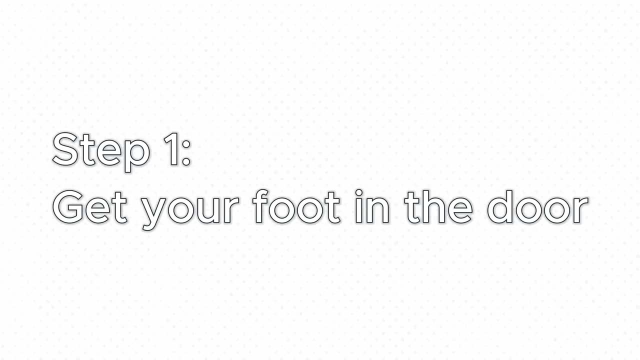 no AI or machine learning experience and still want to become one. you got to play smart and be strategic, So this is what you're going to do. First, start anywhere. You got to get your foot in the door. Don't just wait around waiting for the perfect AI or machine learning role to appear. 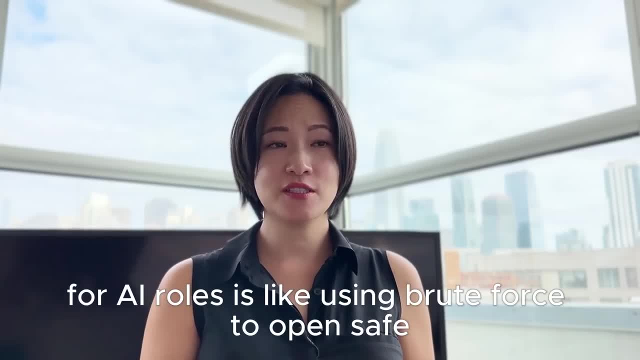 magically Competing with the PhDs for AI roles is like using brute force to open the safe. Try becoming any kind of engineer, full stack, iOS, web world or whatever you want to be. If you're not sure what you want to be, you can start anywhere. 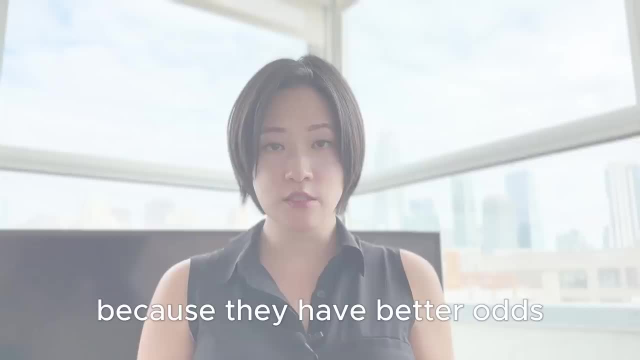 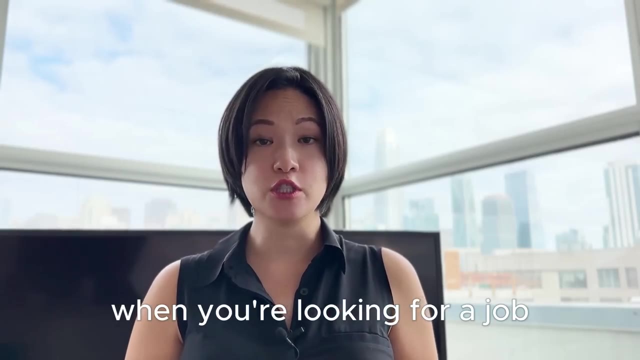 Whatever you pick because they have better odds. The sooner you're employed, the sooner you start gaining real life industry experience, which is what counts the most when you're looking for a job. According to the 2023 future of jobs report, number one thing that companies care about is your. 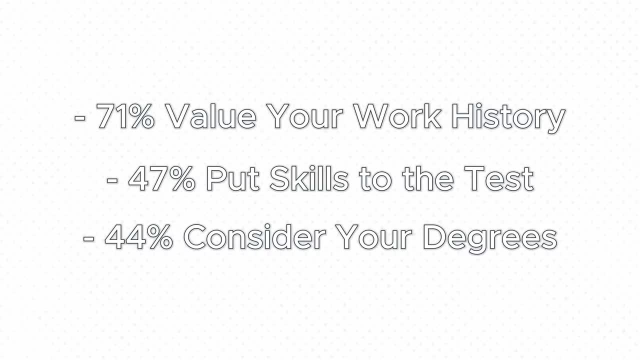 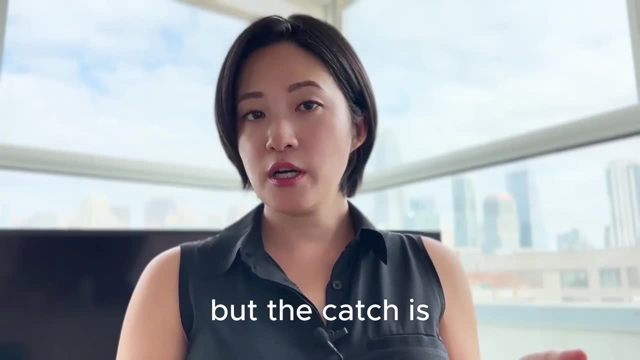 past work. Second, they test your skills. Then third, they check your degrees. This means if you don't have prior work experience, you would need to ace your coding interview. But the catch is, if you can't even pass the resume screening, you're not going to be able to get a job. So 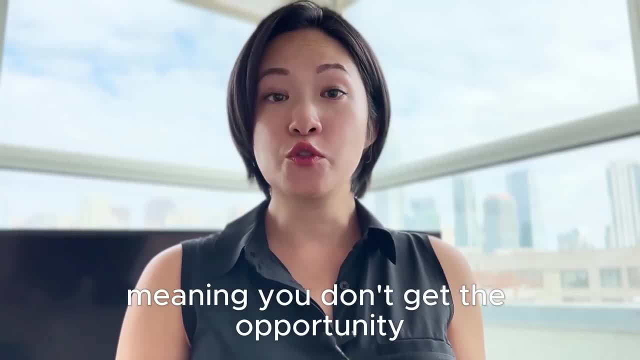 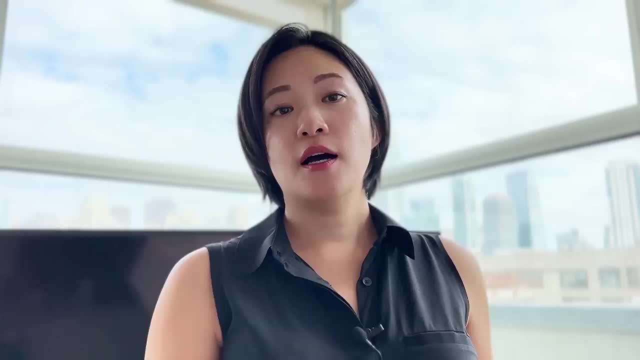 you won't even get an interview, meaning you don't get the opportunity to demonstrate your coding abilities, And I've been there. Before landing my previous role at WhatsApp, I applied for over 300 jobs and got less than a dozen interviews, And that was a relatively active. 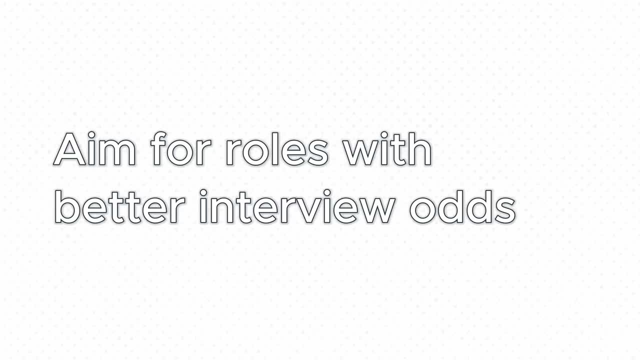 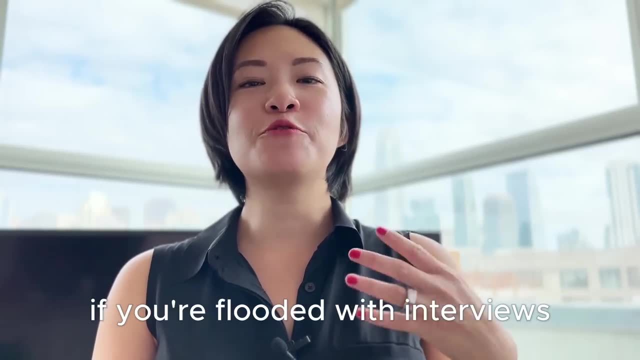 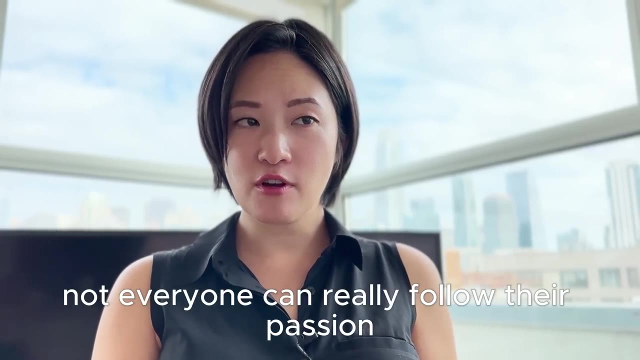 job market. So aim for roles with better interview odds. If your interviews are scarce, go for less competitive roles. And I mean, of course, if you're flooded with interviews, you go for the exciting roles. But in this tough job market, not everyone can really follow their passion. 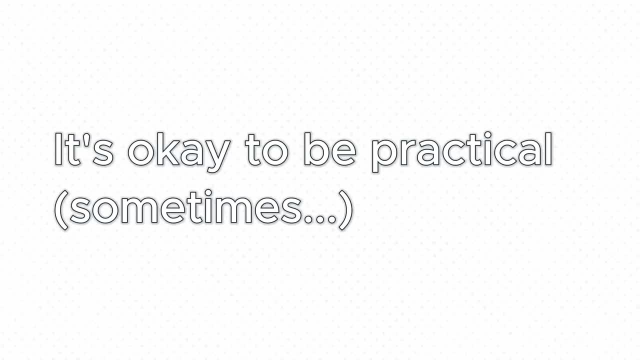 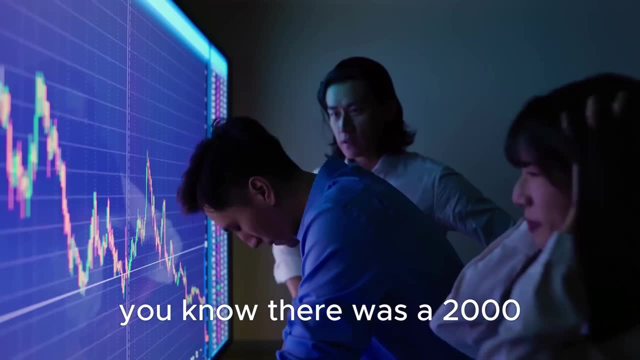 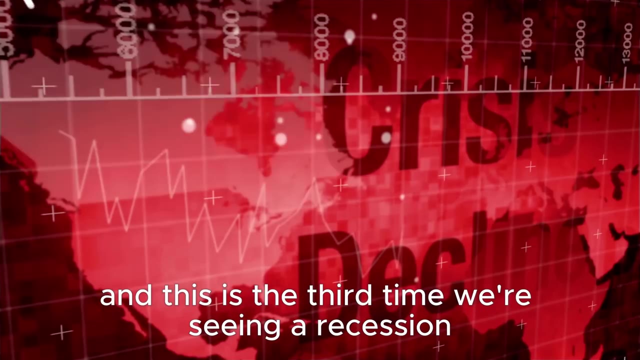 So when times are tough, you operate in a more practical mode, and that's okay. And I say this because this is the third recession I have seen personally. You know there was a 2000 dot com crash and then the 2007 aid financial crisis or the housing crashes, And this is the third time. 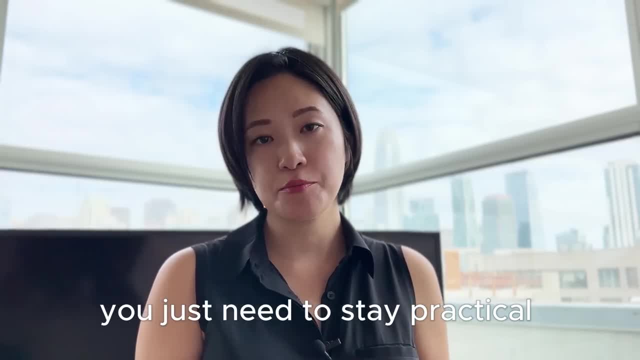 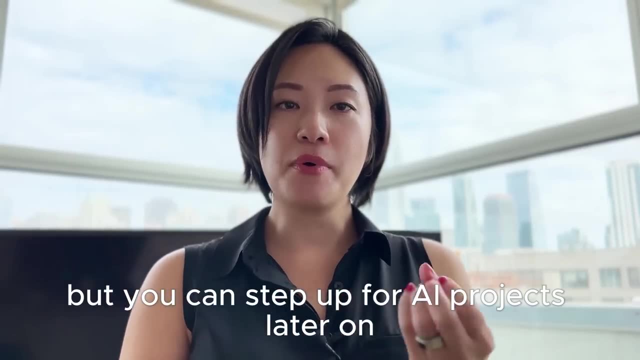 that it's happened, And so the work is to only get better at what you actually need to do. And then you're forced to get into the business world, And it's not really just an irritable situation. It's more of a crisis, It's a shoreline. You have to be prepared to be in your 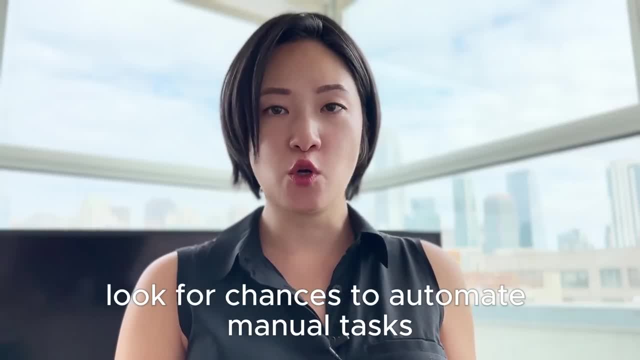 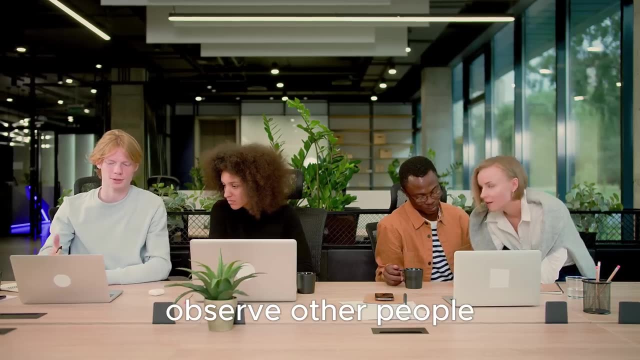 own world, And you know there are times where you might be under a lot of pressure because it's been a bit of a big year and you're just finished a massive year, And so it's your next step to identify and see where you need to go after that. But for now you just need to stay practical At 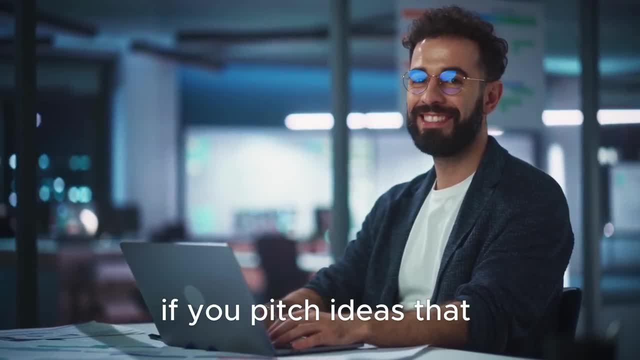 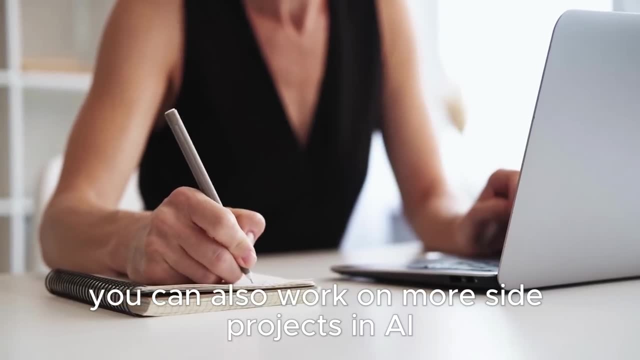 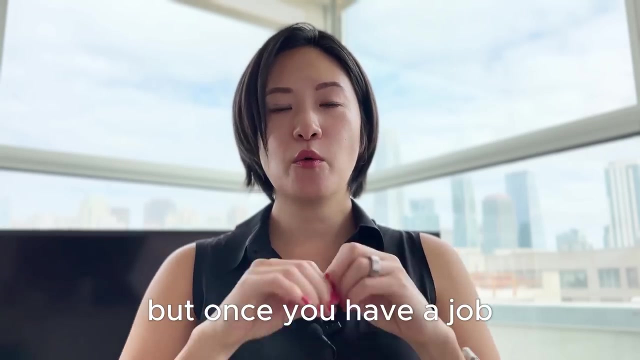 way into the world of ai. if you pitch ideas that actually help people at your workplace, most likely your bosses are going to love it. you can also work on more side projects in ai. now i don't necessarily encourage people to work on side project to get a job, but once you have a job you can work on side. 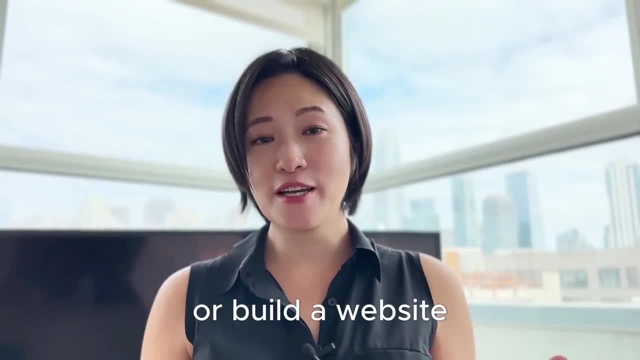 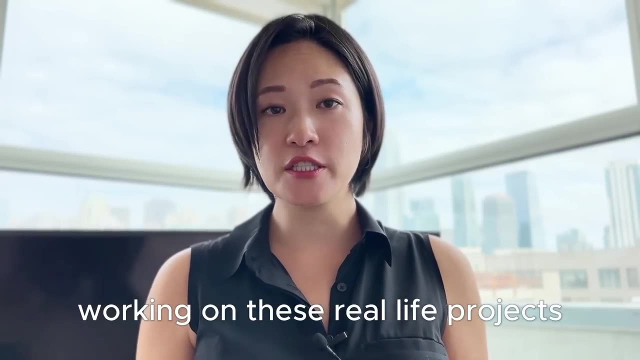 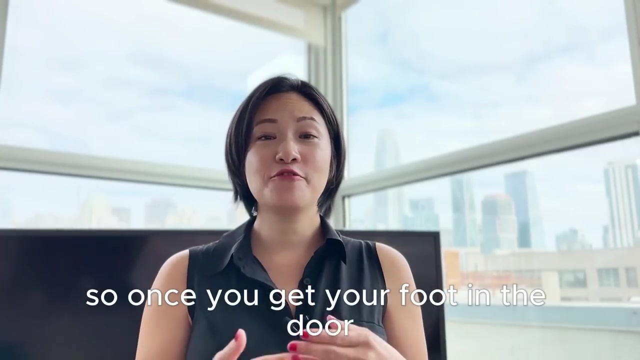 projects, launch an app in the app store or build a website, but with real users. so you build your portfolio and experience working on these real life projects. because, remember the number one thing- companies are looking for prior experience. so once you get your foot in the door, it's much.